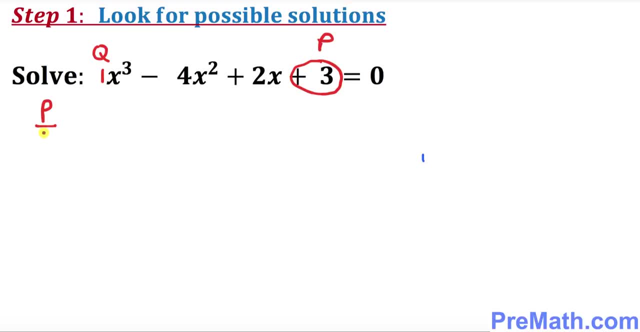 what we got right now: p over q is going to be how much, 3 over 1, which is going to give you what 3.. So our possible solutions going to be what it's going to be: a positive 1, negative 1, positive 3, and what negative. 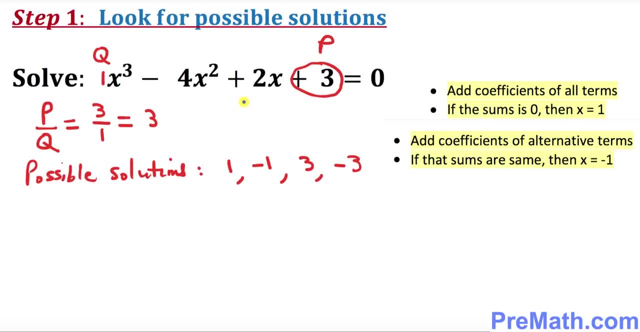 3.. However, if you have watched my previous videos, those videos state what? that if you add all these coefficients- this coefficient, this one, this one and these coefficient- if you add them up, then there's: if their sum is equal to 0, then one of the solution is going to be 1 x equal to 1.. As you can. 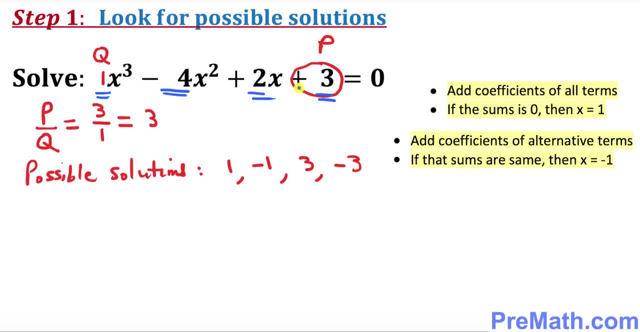 see that when you add these coefficients they do not yield 0. So that means x equal to 1 is not going to be our negative 1.. So that means x equal to 1 is not going to be our negative 1.. So that. 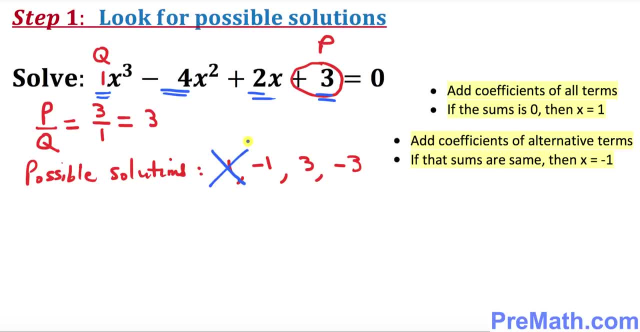 means x equal to 1 is not going to be our negative 1.. So that means x equal to 1 is not going to be our solution. So we're going to rule out this thing. So one is not our solution. The other one rule was: 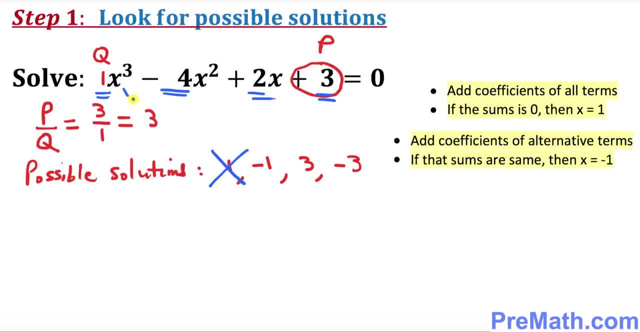 what if you add these alternative numbers, alternative coefficient, this one and these ones, this 1 and 2 give you what? 3 and this negative 4 and 3 give you negative 1.. Since these two numbers are not same, so that means our next x equal to negative one is not our solution as well. 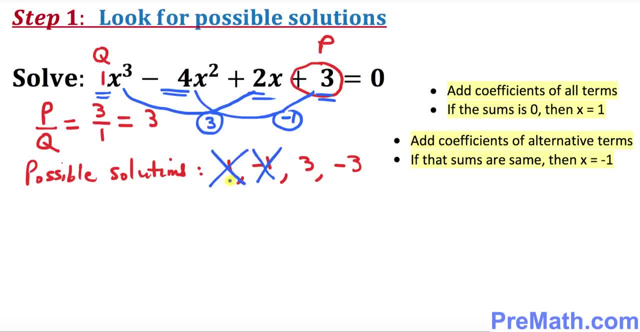 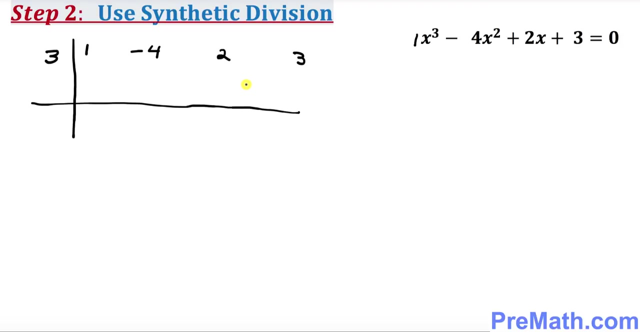 so we ruled out two possible these numbers. so one can't be our solution and negative one can't be our solution. so now we are our pinning our hope on only these one three and negative three. so now let's go ahead and try three. so in step two we're going to be using synthetic division. i put down: 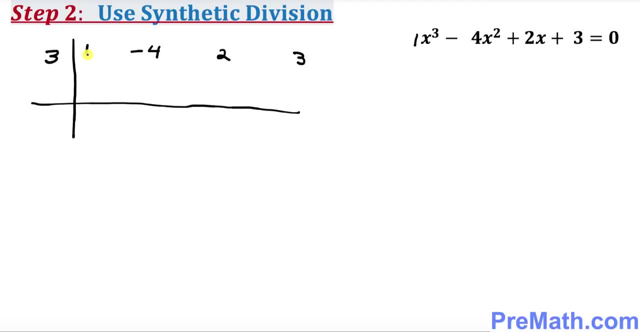 all these coefficients right up here, one negative four, two and three, and the number that we're going to be testing is x equal to three, so let's see what happens. so, first of all, i want to make sure you leave that one as it is. one is not. 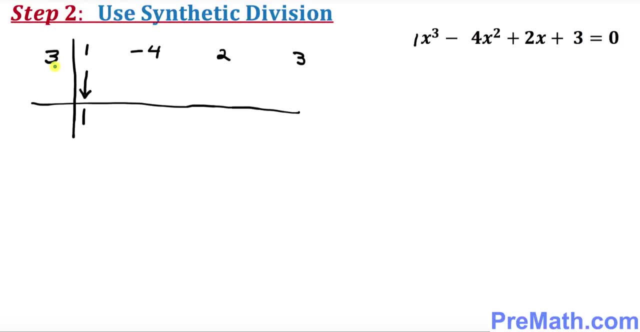 going to change now. the next thing, what i want you to do is i want you to multiply three times one. that's going to give you what three? you add them up right here, so that's going to give you negative one once again. i want you to multiply three diagonally with the negative one. 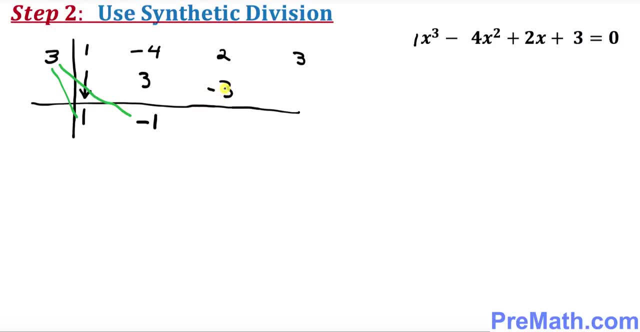 that's going to give you negative three. so that turns out to be what negative one when you add these two numbers. so next thing again: multiply three, uh, with negative one diagonally. again, that's going to give us what negative three, three and negative three is going to give us what zero. zero is our remainder. always remember when. 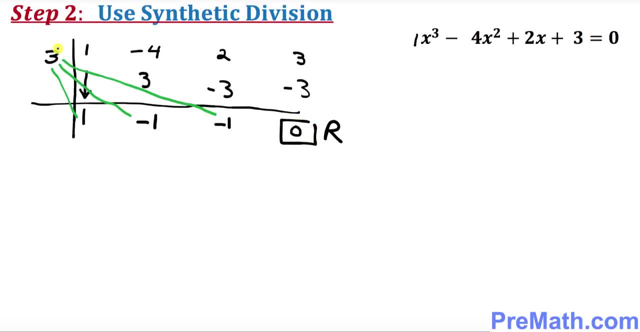 the remainder is zero. that means this: whatever number three is, of course, this is one of our solutions. so we figured out. that means what x equals to three is one of our solutions. just keep in your mind. so now, next thing, what we want to do is: i want. 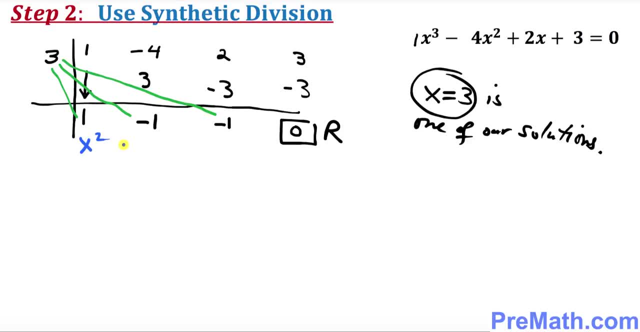 you to just now. this is going to become what? x square? this is x, and this term, this number, is without x. so that's going to give us what? so this is going to become one x square minus one x, and then this is negative one, equal to what? zero? and now we're gonna solve for x, this quadratic equation. so 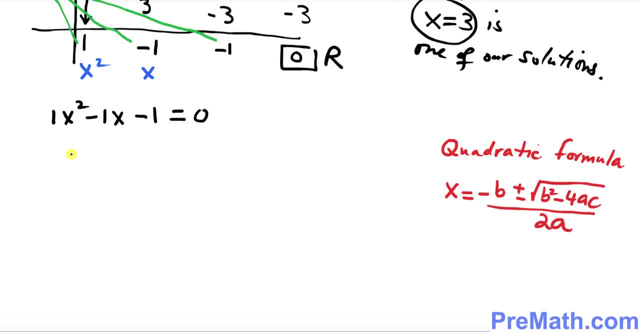 so now we're gonna be using this quadratic formula that you can see on the right hand side. so in this case, in this quadratic equation, a equals to one, b equals to negative one and c equal to negative one as well. so x equal to minus, b means negative time, negative one plus. 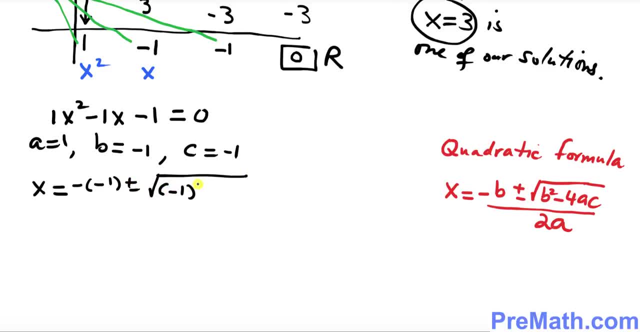 b square is going to be what negative. one square minus four times a is one. c is negative. one divided by two times a is one. so the next is going to become what this is going to. what negative i is going to be is going to be negative. two over a power n i Ke bet several times. 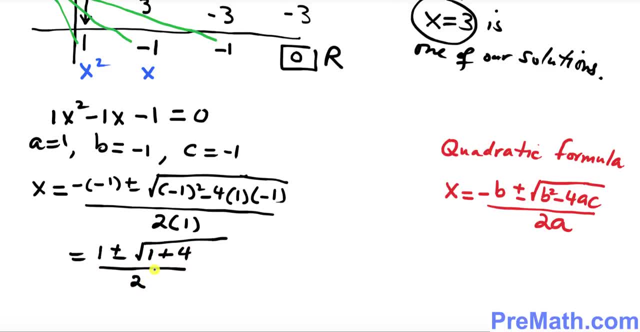 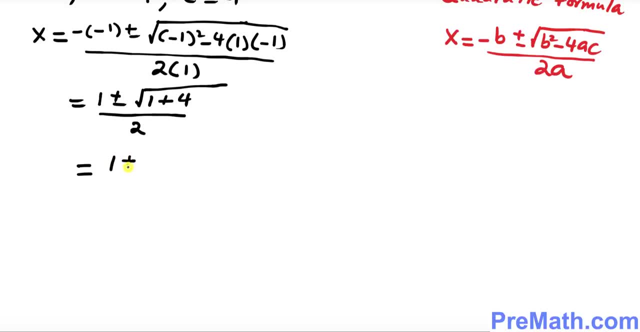 at a time is going to be this negative, so that's going to be negative three times a minus 4 j, quindi plus b times b times b. our answer here is equal to negative, or there's an opposite, positive to a divided by three, divided by two, negative. so here's the whole thing. we're not going to just fix it just like the otheraaaaa. 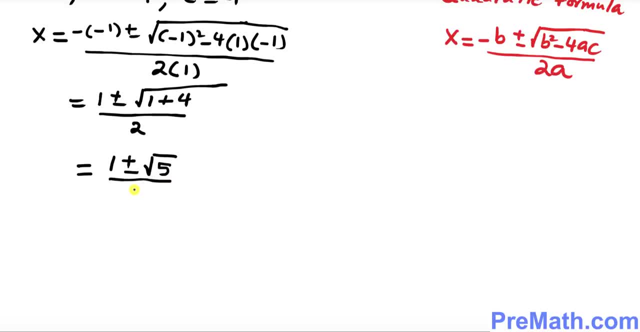 rule. we're going to complete that like thatğimiz, just like this, looking at iteeeeeee 2, so we can split this thing up: 1 plus 5 over 2. this is one of the solutions: x equal to this one and the other one is going to be x equal to 1 minus square. 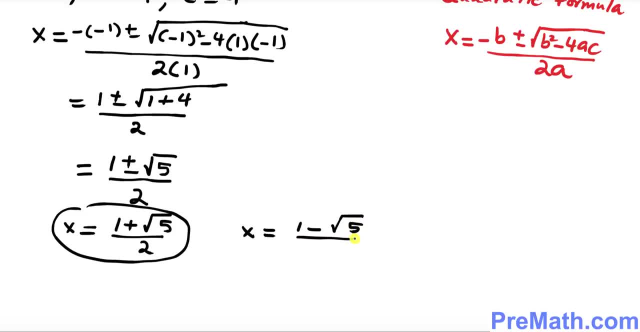 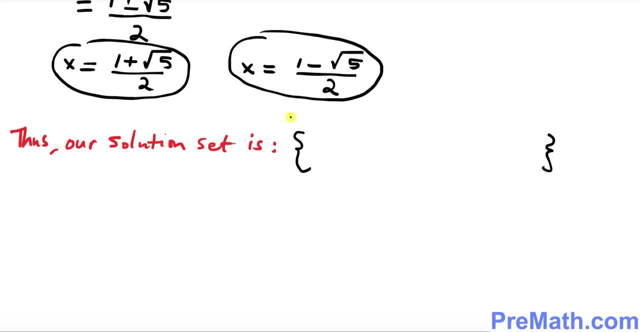 root of 5 divided by 2. these are two solutions. thus our complete solution set is going to be what? now? you know that at the previous step we already figured out: x equal to 3 is one of our solutions. the next are what? 1 plus square root of 5. 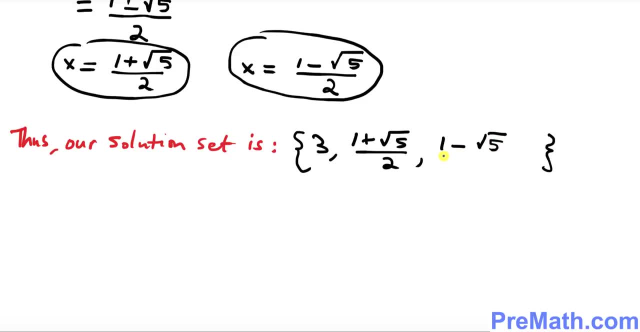 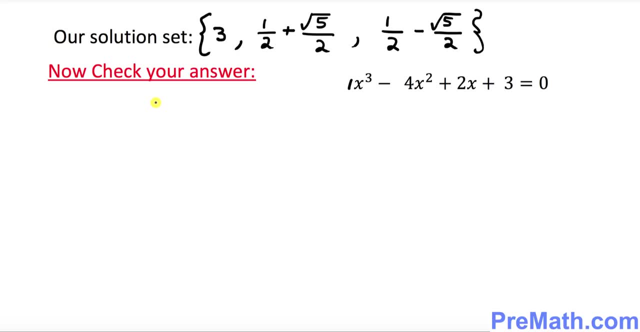 minus square root of 5 over 2. so these are our two solution, three solutions, and our final step is this thing: the final step, we want to check our answer. so the very first step I want you to do is I want you to add our whatever three. 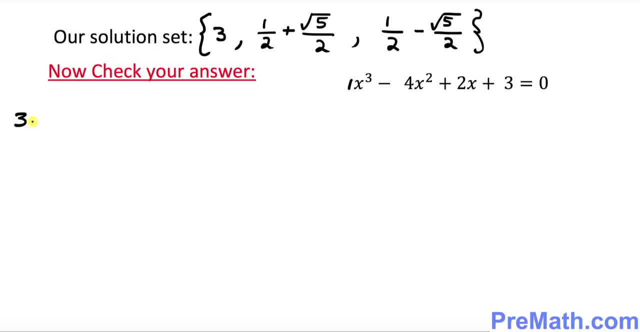 solutions. we got what. our three solutions are what? 3 plus 1 over 2, plus square root of 5 over 2, and then plus 1 over 2 minus square root of 5 over 2. ask yourself: is it equal to minus B over a? now you might be wondering what.